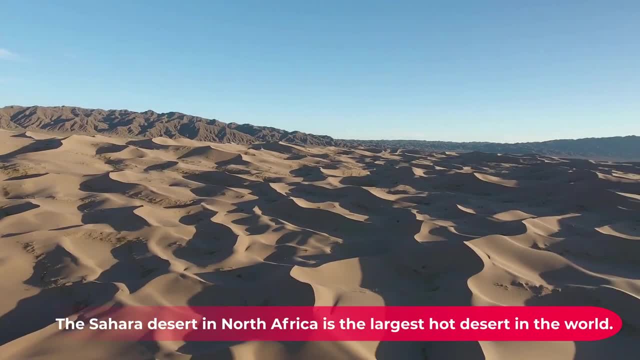 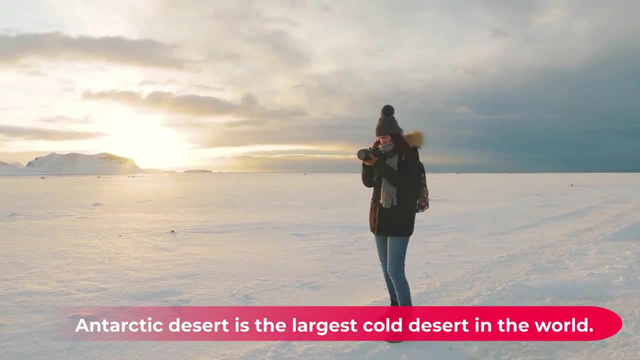 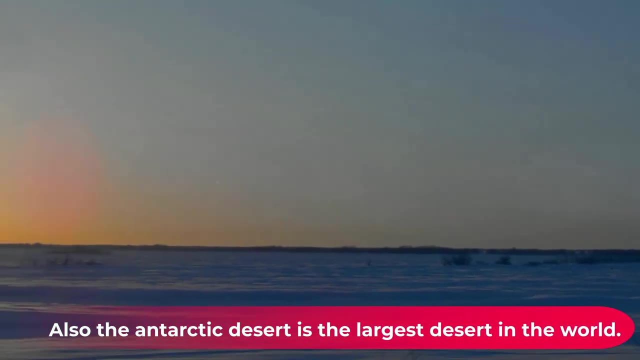 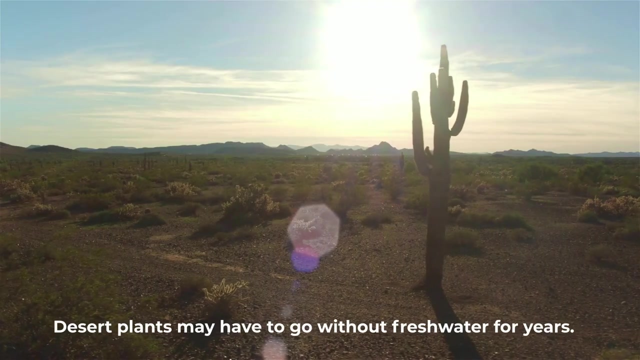 The Sahara Desert in North Africa is the largest hot desert in the world. The Antarctic Desert is the largest cold desert in the world. Also, the Antarctic Desert is the largest desert in the world. Desert plants may have to go without fresh water for years. 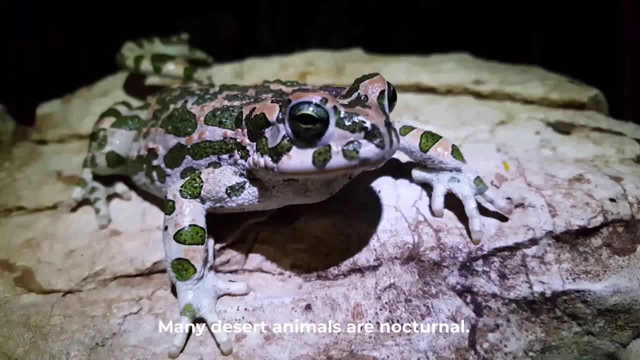 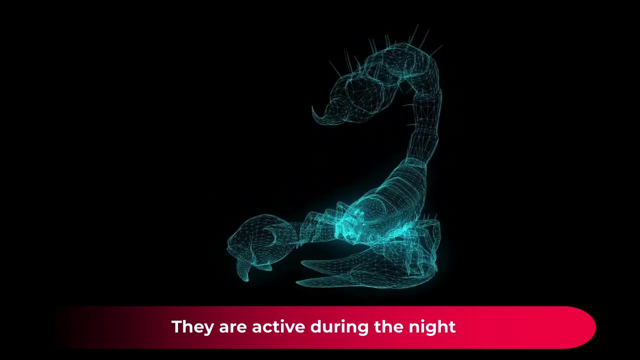 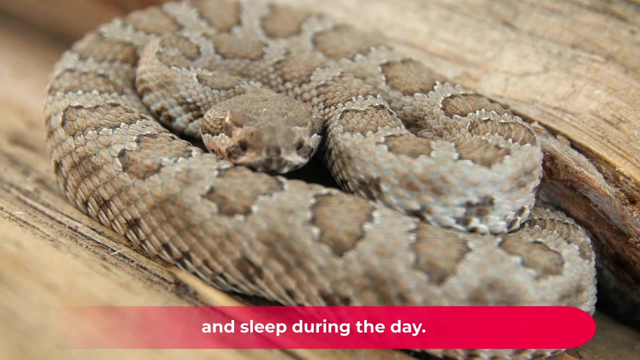 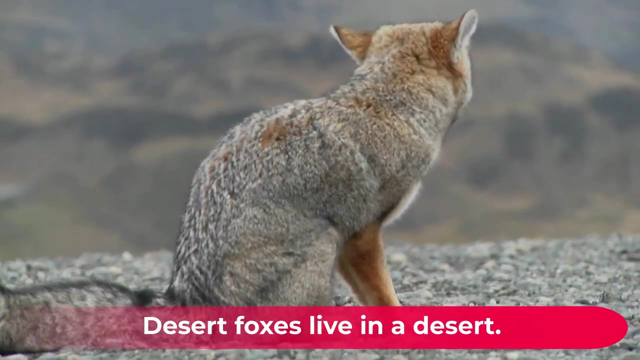 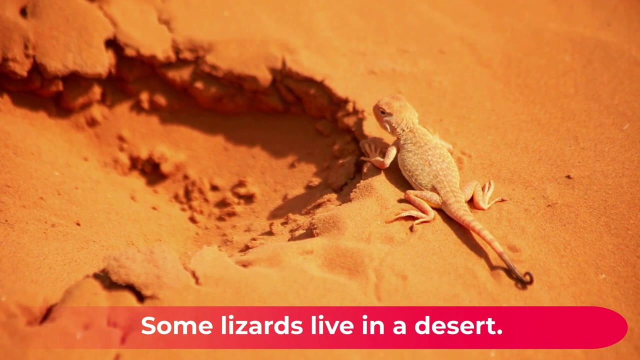 Many desert animals are nocturnal. They are active during the night And sleep during the day. Desert foxes live in a desert. Some lizards live in a desert. Some lizards live in a desert. Some lizards live in a desert. 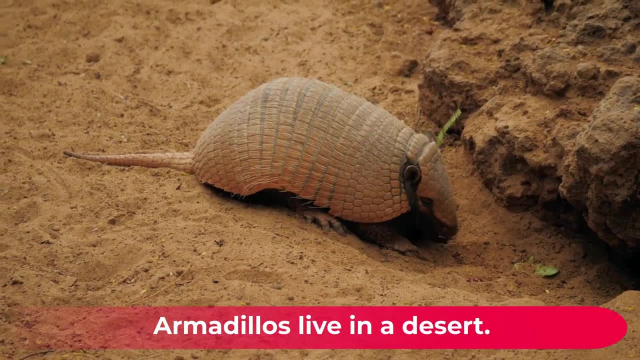 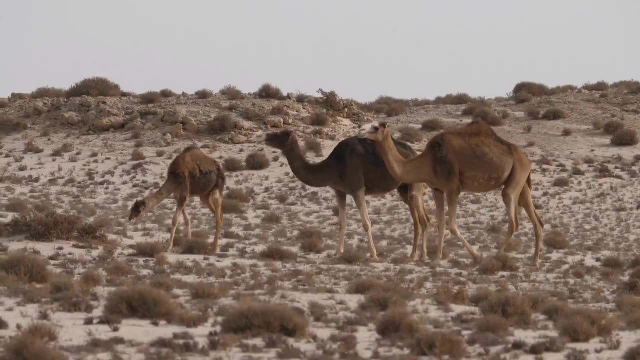 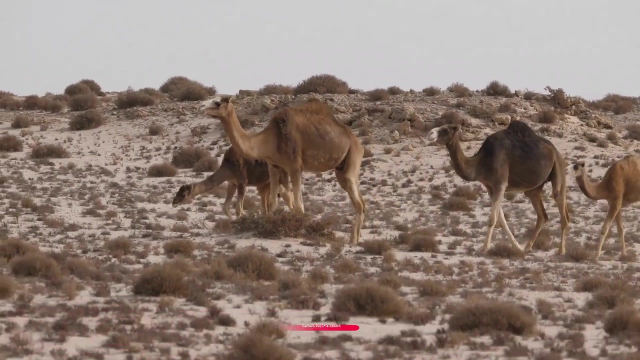 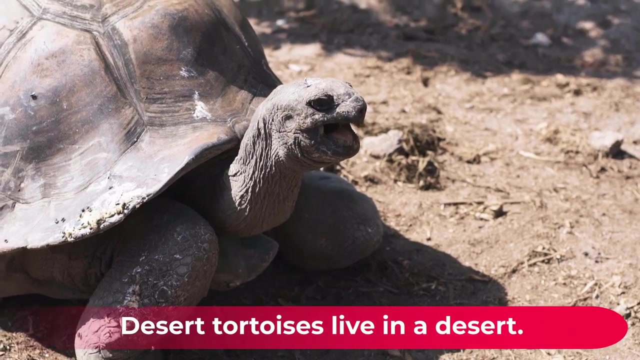 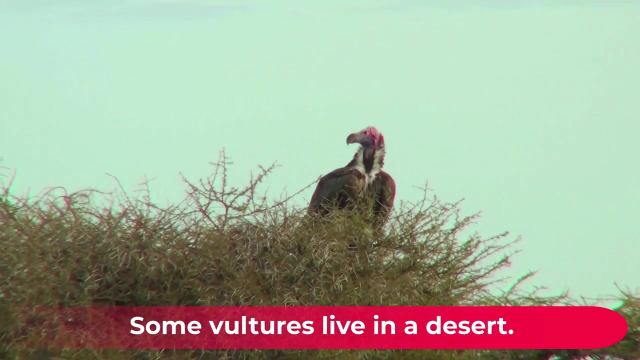 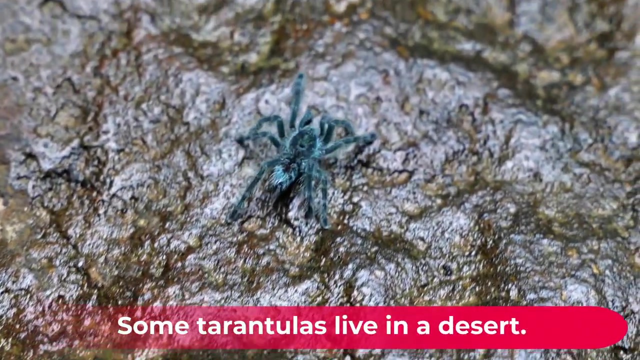 Armadillos live in a desert. Camels live in a desert Desert tortoises live in a desert. Some vultures live in a desert. Some tarantulas live in a desert. Some tarantulas live in a desert. 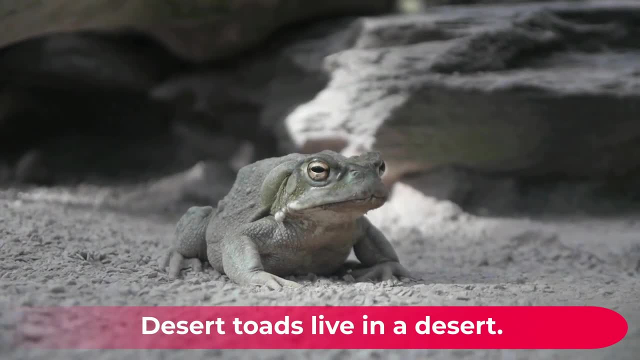 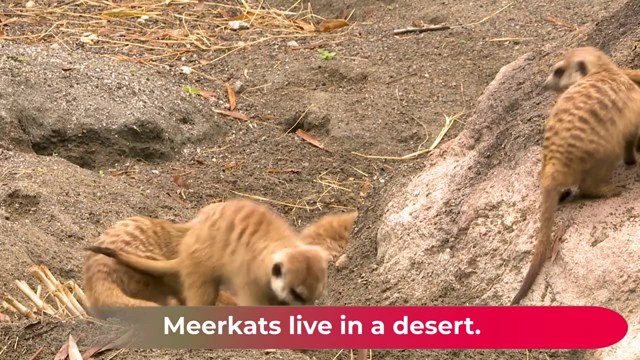 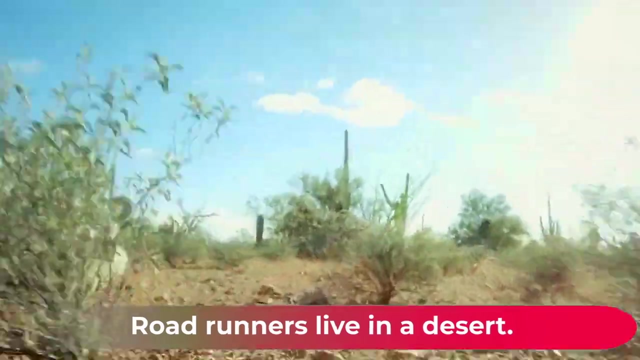 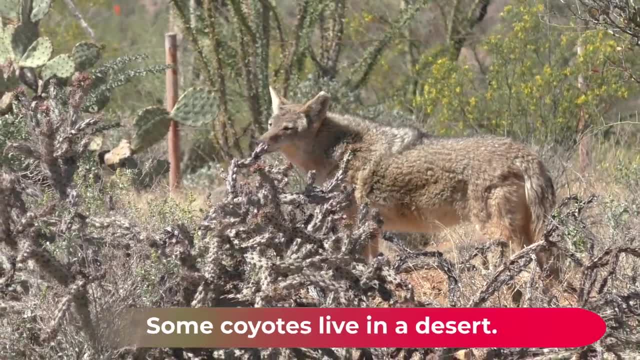 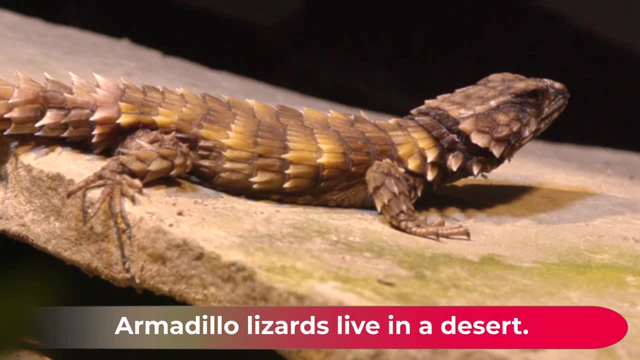 Some coyotes live in a desert. Some coyotes live in a desert. Armadillo lizards live in a desert. Armadillo lizards live in a desert. Armadillo lizards live in a desert. Thorny devils live in a desert. 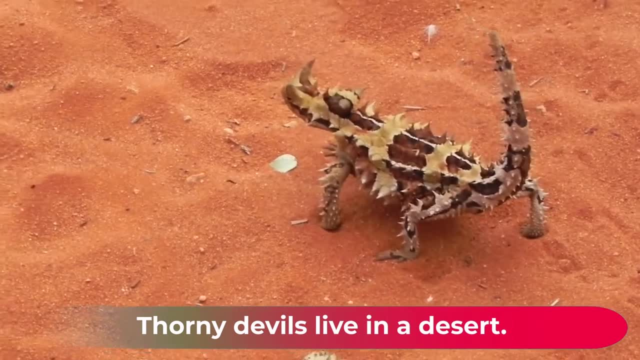 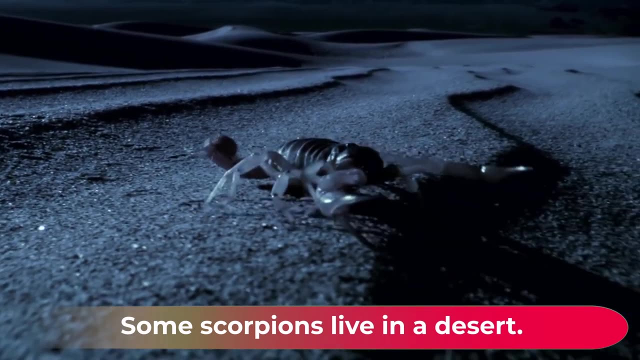